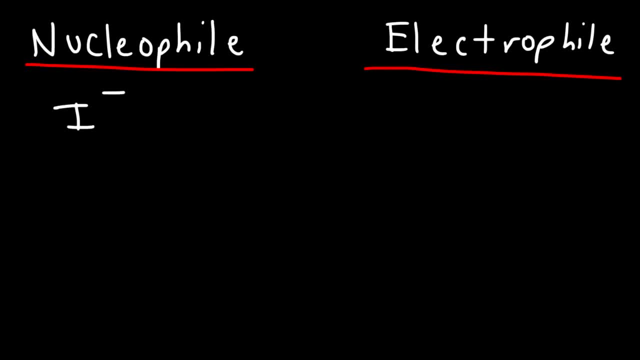 examples of nucleophiles would be iodide: it has a negative charge. Water can behave as a nucleophile. It's attracted to the nucleus, which usually bears a positive charge. Some other examples of nucleophiles include hydroxide that could behave as a nucleophile, Ammonia- that's another. 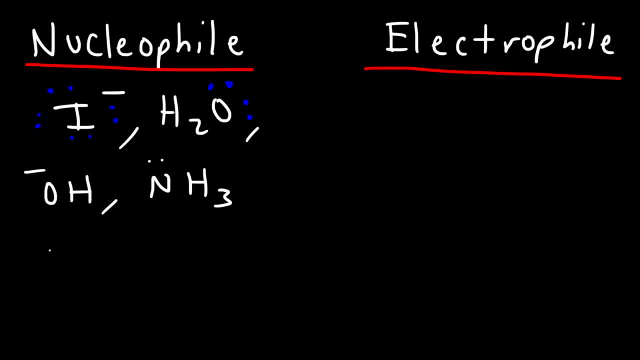 nucleophile Electrophiles usually bear positive charges. They seek out electrons. they love electrons. So H plus is an electrophile, Fe3 plus, that's another one. A carbocation is an electrophile. Some other electrophiles may not have a. 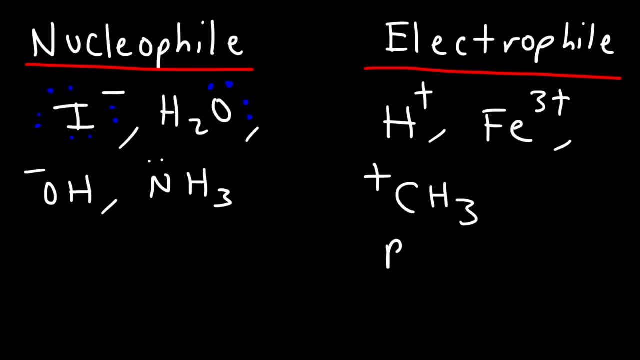 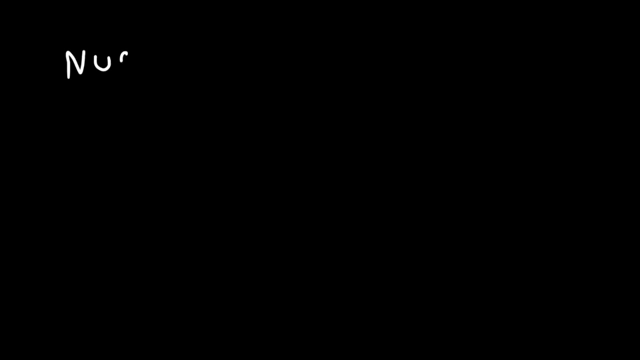 positive charge, but they can accept a pair of electrons. So BH3, FeBr3, AlCl3, all of these can form a nucleophile. They can accept a pair of electrons, And so an electrophile is basically a Lewis acid. A nucleophile is basically a Lewis base. Now, when dealing with the reaction, 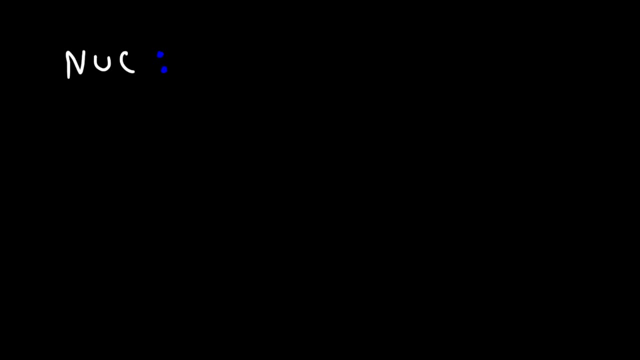 mechanisms between nucleophiles and electrophiles. when drawing the arrow, it's always going to flow from the nucleophile to the electrophile. The arrow represents the direction of the electron flow, So it's going to travel from a region of negative charge. 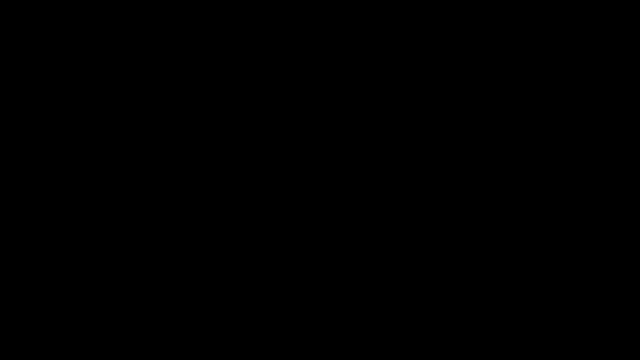 to a region of positive charge. So let me give you some examples. Let's say if we were to put hydroxide with a methyl carbocation. We know that opposites attract. Hydroxide is going to donate a pair of its electrons. 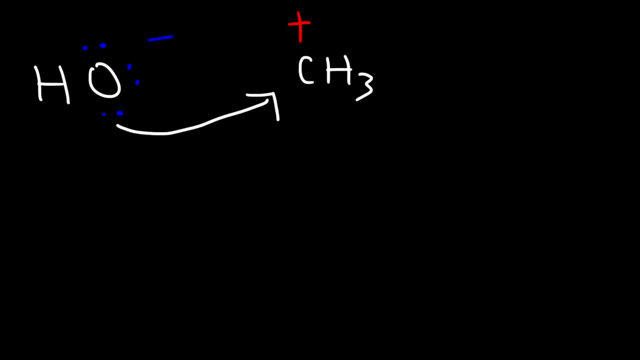 to the carbon atom, And so we're going to get methanol, And now the oxygen has two lone pairs as opposed to three. Now let's say if we had BF3.. It doesn't have a positive charge, it's neutral, And so this is going to be the electrophile. Now let's. 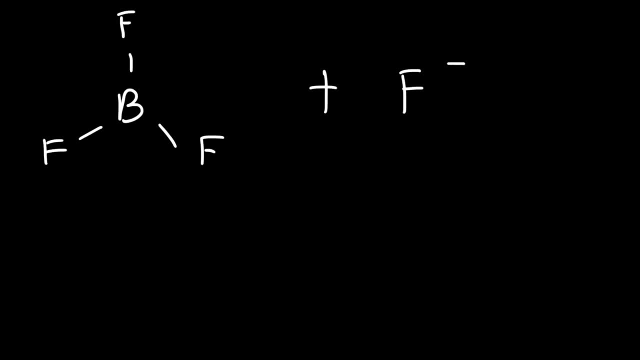 react it with a nucleophile, in this case fluoride. It's electron-rich, it has a lot of lone pairs, And so the nucleophile is going to attack the electrophile. And so this is a typical Lewis acid-base reaction. And 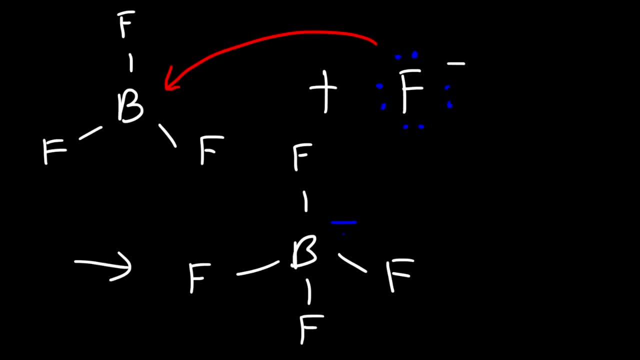 now the boron carries the negative charge. Now here's a question for you: What about a ketone? Would you say it's a ketone, Or would you say it's a ketone? Would you say it's a ketone? 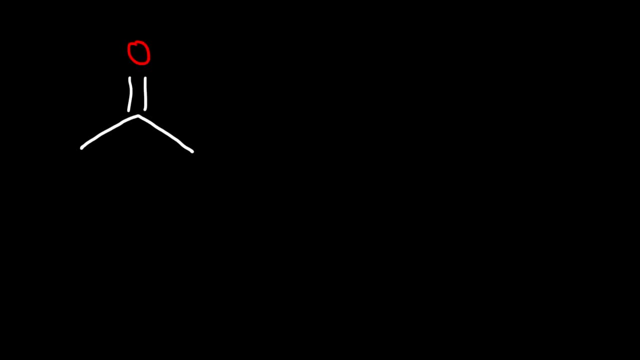 Would you say it's a ketone? Would you say it's a nucleophile Or would you say it's an electrophile? Think about it. I'm going to give you a few minutes to find the answer to that question. Is a ketone an electrophile or is it a nucleophile? 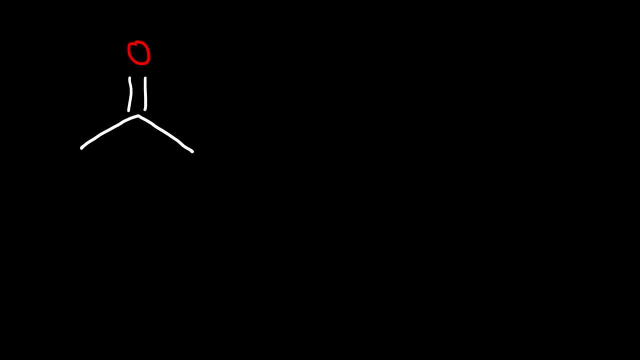 Technically, it depends on what is attacking it or what's around it. Under basic conditions, the ketone tends to behave more as an electrophile. Under acidic conditions, it tends to behave more as a nucleophile. Now, the reason why it can behave as both is because, if you draw the resonance structure, 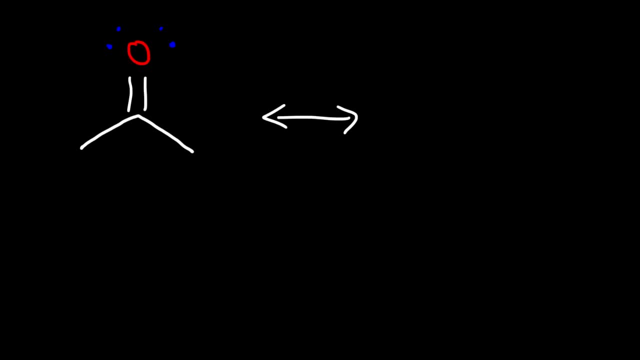 of this ketone, you'll see that it has a region that's nucleophilic and a region that's electrophilic. So if we take this pi bond and move those two electrons to the oxygen atom, we're going to get this resonance structure. 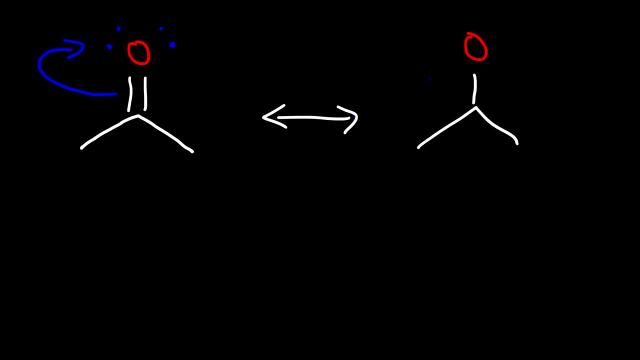 And so the oxygen is going to carry three lone pairs now and it's going to have a negative charge. The carbon atom has a positive charge. So, as you can see, the carbon atom of a ketone that is electrophilic. 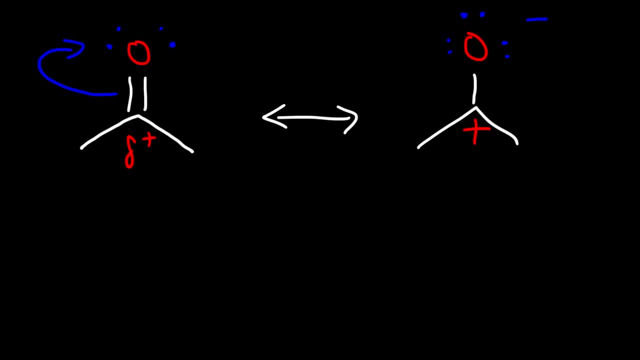 It bears a partial positive charge. The oxygen atom bears a partial negative charge in its original form, And so the oxygen part of the ketone is nucleophilic, The carbon part is electrophilic. So, for example, let's say, if we reacted a ketone with a nucleophile such as I'm going